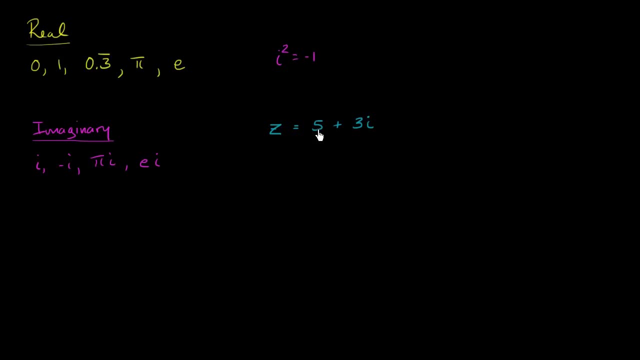 And you might be tempted to add these two things, but you can't. It won't make any sense. These are kind of going in different. Well, we'll think about it visually in a second, But you can't simplify this anymore. 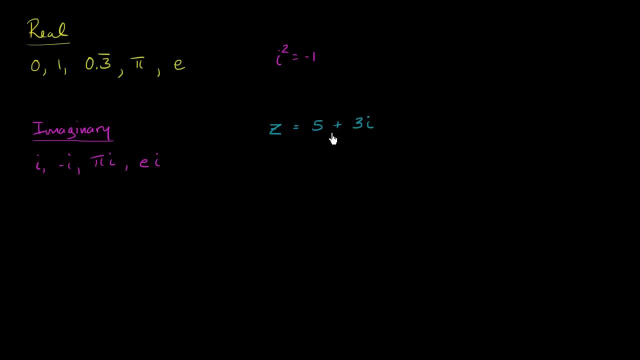 You can't add this real number to this imaginary number. A number like this- and let me make it clear, that's real And this is imaginary- A number like this we call a complex number Complex number. It has a real part and an imaginary part. 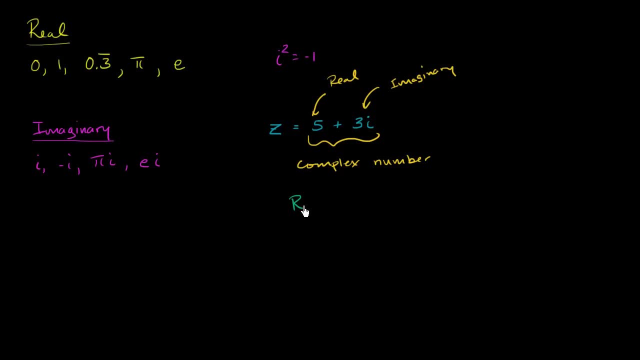 And sometimes you'll see notation like this, where someone will say: well, what's the real part, What's the real part of our complex number z? Well, that would be the 5 right over there. And then they might say: well, what's the imaginary part? 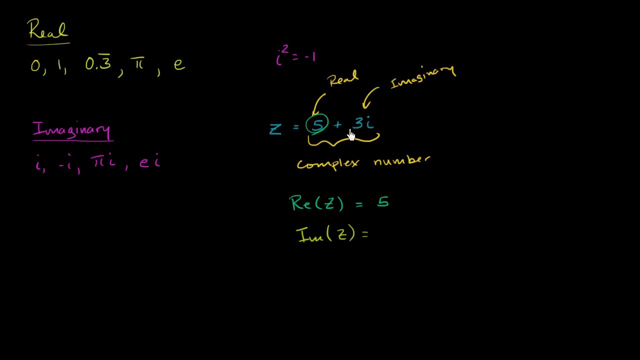 What's the imaginary part of our complex number z, And then typically the way that this function is defined. they really want to know, well, what multiple of i is this imaginary part right over here, And in this case it is going to be 3.. 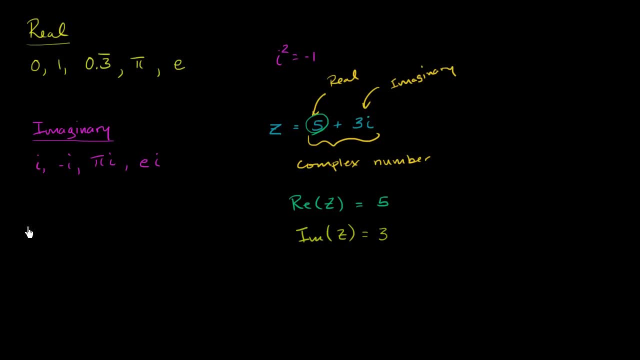 And we can visualize this. We can visualize this in two dimensions. Instead of having the traditional two-dimensional Cartesian plane with real numbers on the horizontal and the vertical axis, what we do to plot complex numbers is on the vertical axis, we plot the imaginary part. 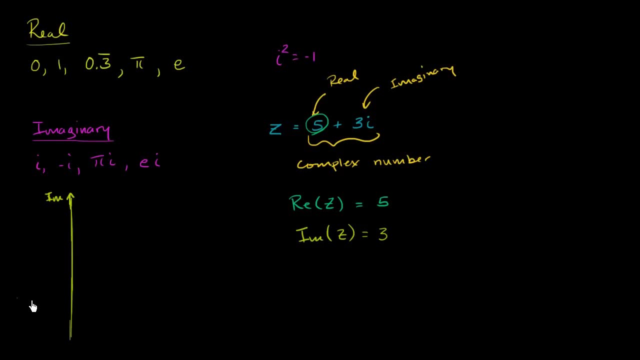 So that's the imaginary part. And then on the horizontal axis we plot the real part. just like that We plot the real part. So for example, z right over here, which is 5 plus 3i, the real part is 5.. 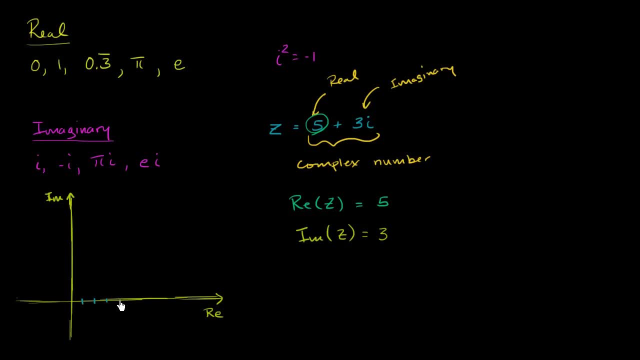 So we would go 1,, 2,, 3,, 4,, 5.. That's 5 right over there. The imaginary part is 3.. 1,, 2,, 3.. And so, on the complex plane, we would: 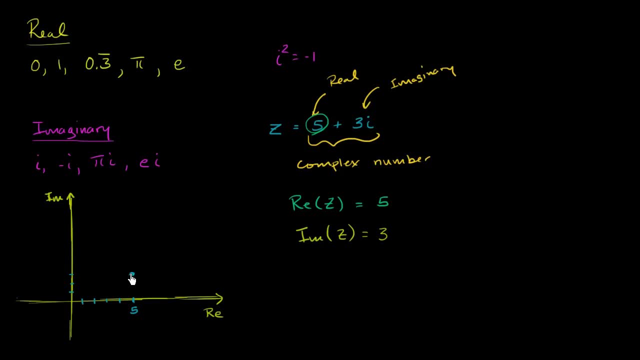 visualize that number right over here. This right over here is how we would visualize z on the complex plane. It's 5, positive 5 in the real direction, positive 3 in the imaginary direction. We could plot other complex numbers. Let's say we had the complex number a, which is equal to. 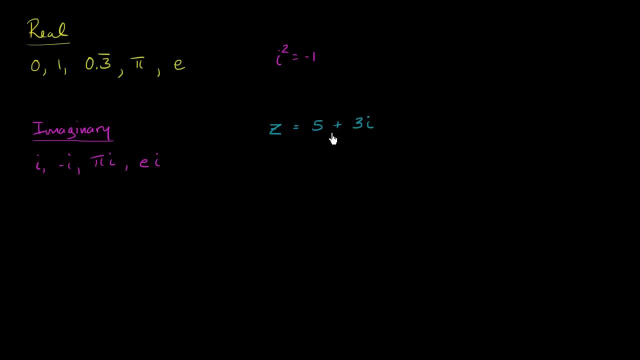 You can't add this real number to this imaginary number. A number like this- and let me make it clear, that's real And this is imaginary- A number like this we call a complex number Complex number. It has a real part and an imaginary part. 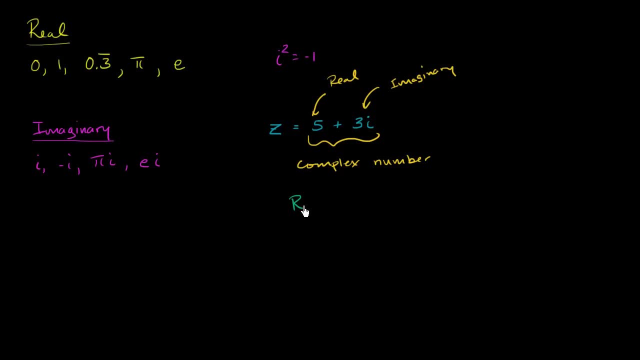 And sometimes you'll see notation like this, where someone will say: well, what's the real part, What's the real part of our complex number z? Well, that would be the 5 right over there. And then they might say: well, what's the imaginary part? 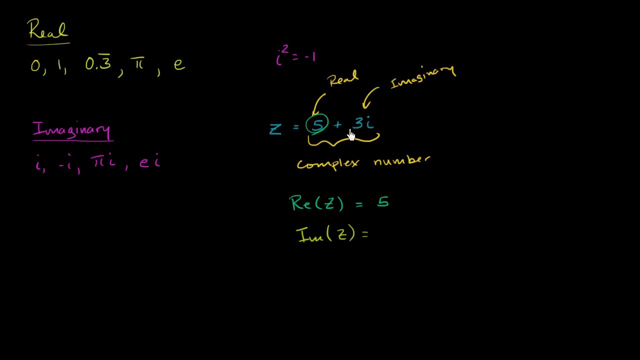 What's the imaginary part of our complex number z, And then typically the way that this function is defined. they really want to know, well, what multiple of i is this imaginary part right over here, And in this case it is going to be 3.. 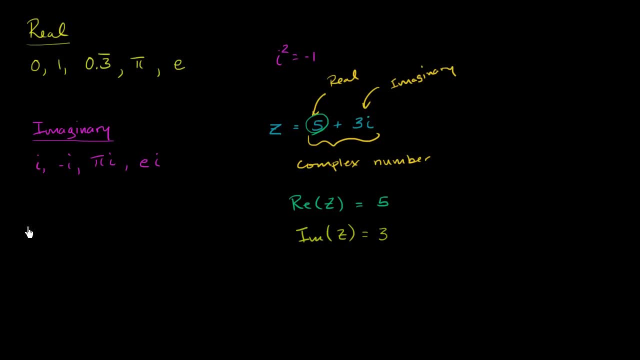 And we can visualize this. We can visualize this in two dimensions. Instead of having the traditional two-dimensional Cartesian plane with real numbers on the horizontal and the vertical axis, what we do to plot complex numbers is on the vertical axis, we plot the imaginary part. 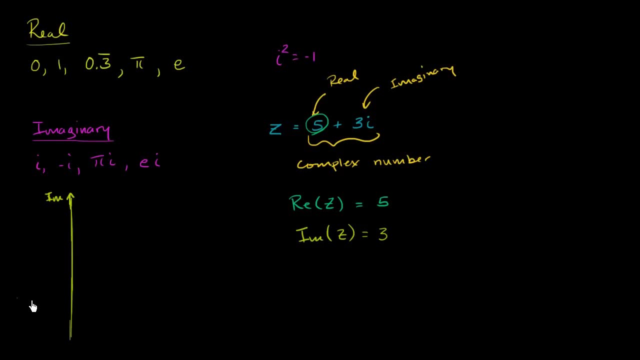 So that's the imaginary part. And then on the horizontal axis we plot the real part. just like that We plot the real part. So for example, z right over here, which is 5 plus 3i, the real part is 5.. 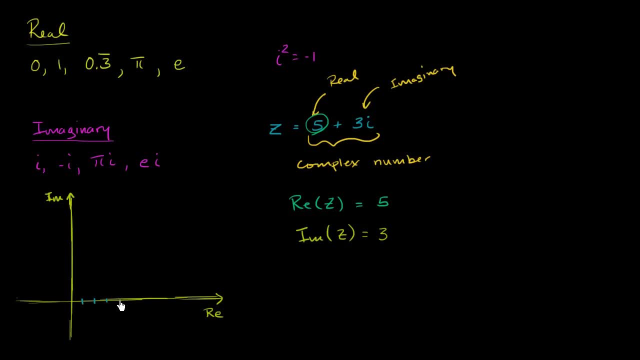 So we would go 1,, 2,, 3,, 4,, 5.. That's 5 right over there. The imaginary part is 3.. 1,, 2,, 3.. And so, on the complex plane, we would: 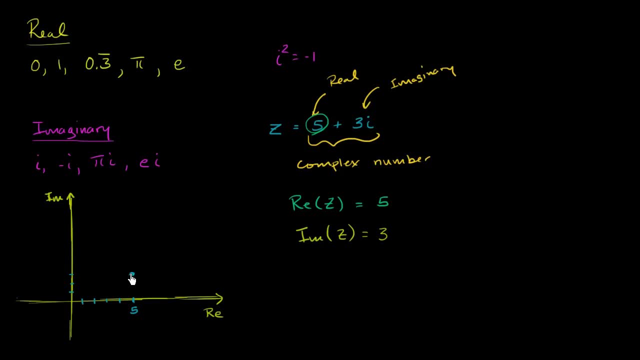 visualize that number right over here. This right over here is how we would visualize z on the complex plane. It's 5, positive 5 in the real direction, positive 3 in the imaginary direction. We could plot other complex numbers. Let's say we had the complex number a, which is equal to.